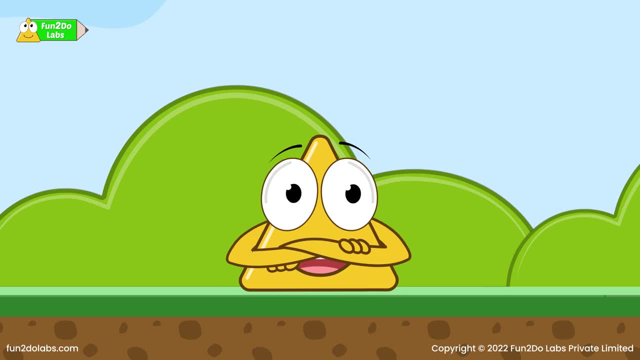 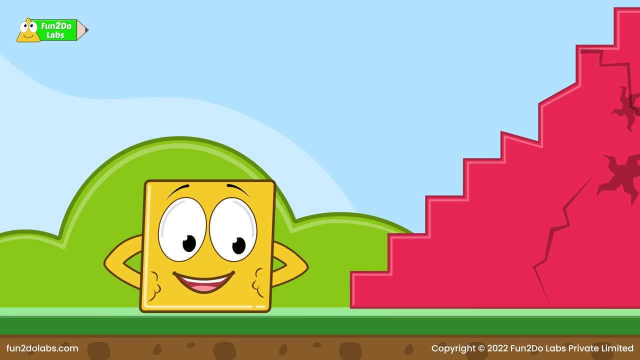 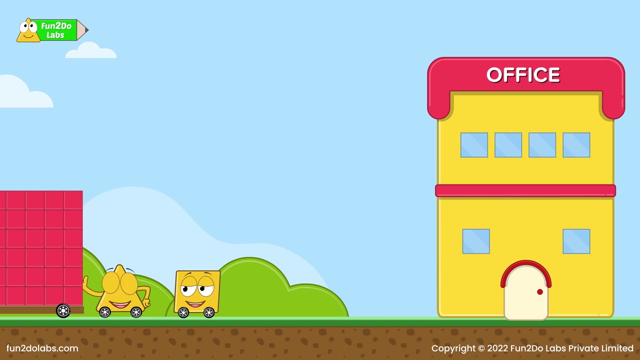 Being flat objects, they will provide good support and will be easy to climb. What do you think? Squero loves the idea and is all excited. First they remove the old steps, Then, one by one, they get the bricks close to the office to make the new steps. 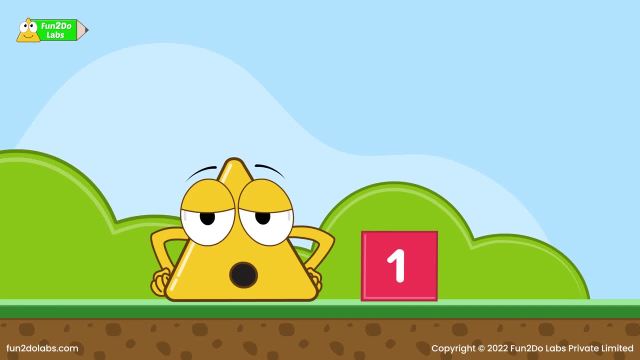 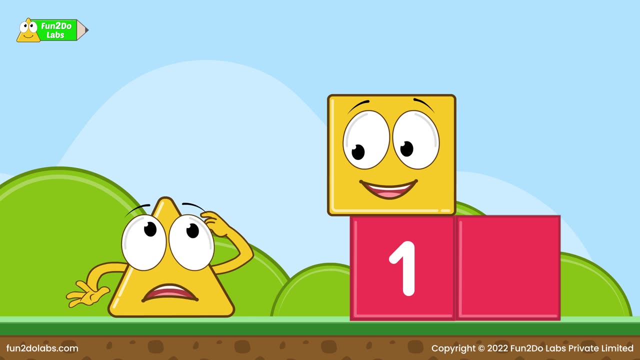 All right, Here I place one brick to form the first step, And here I place another brick next to it to form the next step. Squero, if you place the bricks at the same level, how will you reach the top floor? 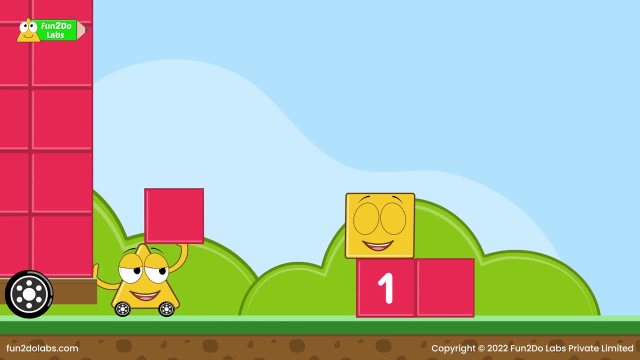 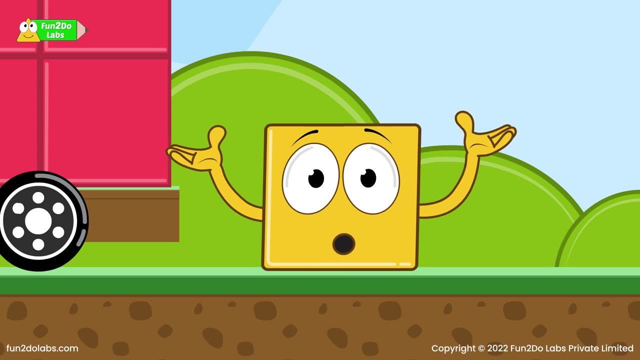 We will have to increase the height of the steps. He picks a new brick and places it over Squero's brick to form the second step, And that means every time we make the next step we could just increase the number of bricks by one right. 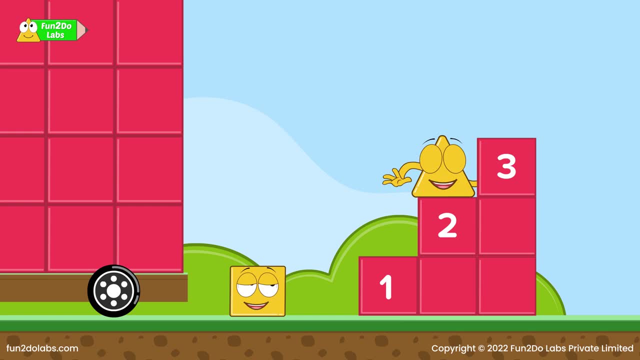 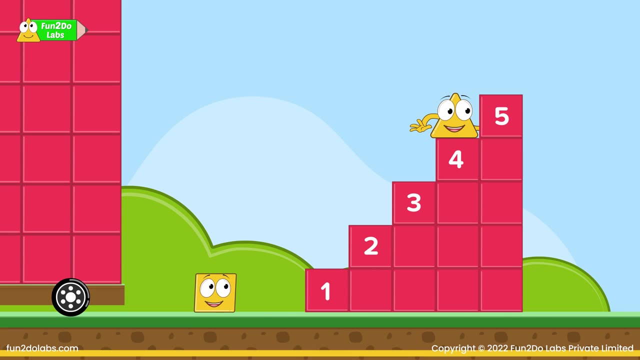 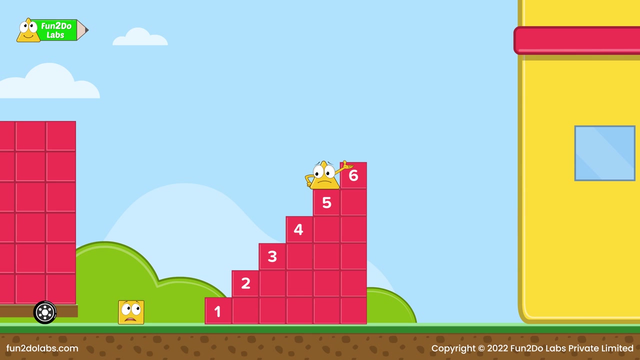 Says Squero Trio agrees with him. Soon they build the third step using three bricks, The fourth step using four bricks, The fifth step using five bricks And the sixth step using six bricks. Oh no, we cannot reach the top floor roof yet. 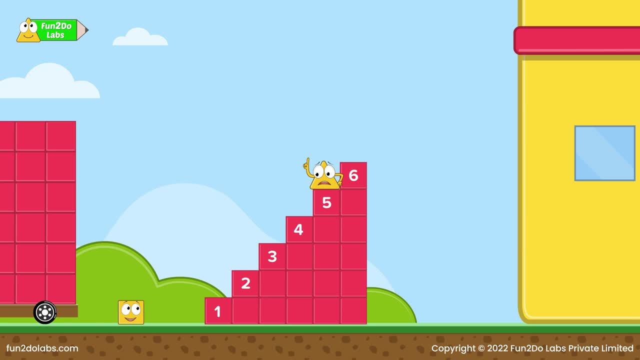 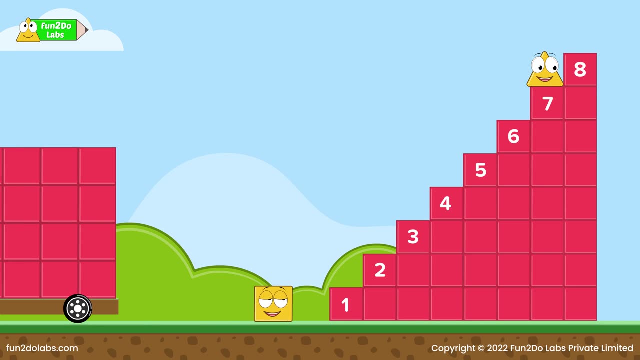 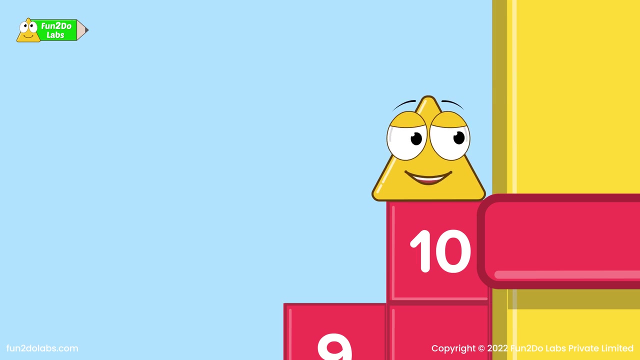 We will need more steps, Says Trio. They build the seventh step using seven bricks, The eighth step using eight bricks, The ninth step using seven bricks, The ninth step using nine bricks And finally, the tenth step using ten bricks. Hooray, I can reach the top floor now. 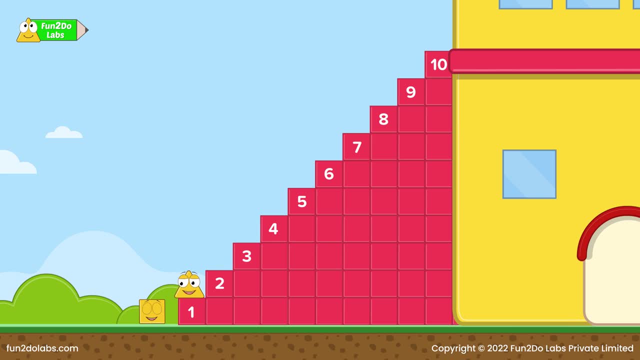 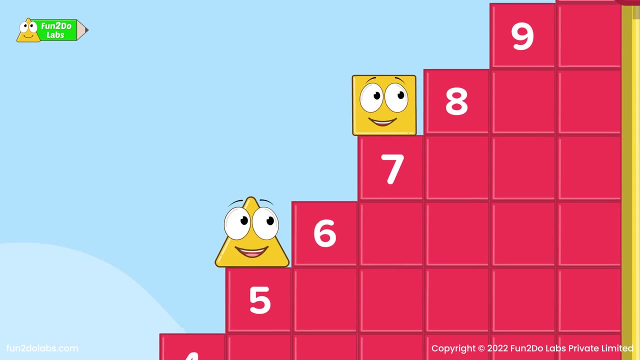 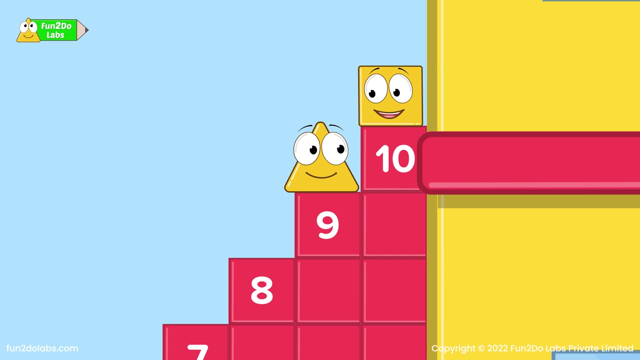 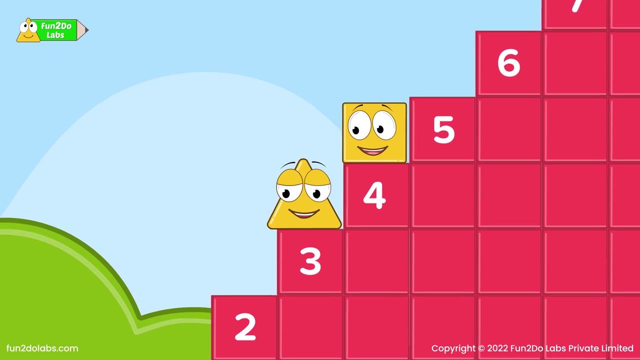 Both excited, they start playing on the steps One, two, three, four, five, six, seven, eight, nine, ten. We count the steps as we go up: Ten, nine, eight, seven, six, five, four, three, two, one. 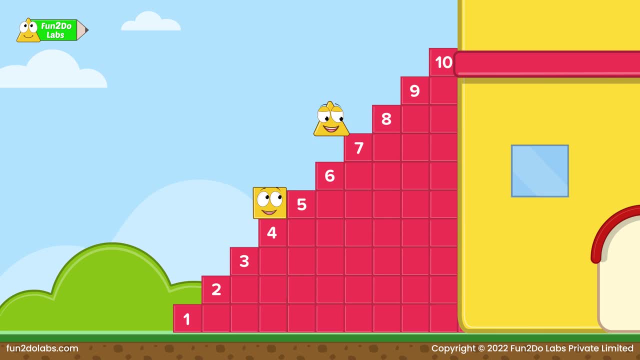 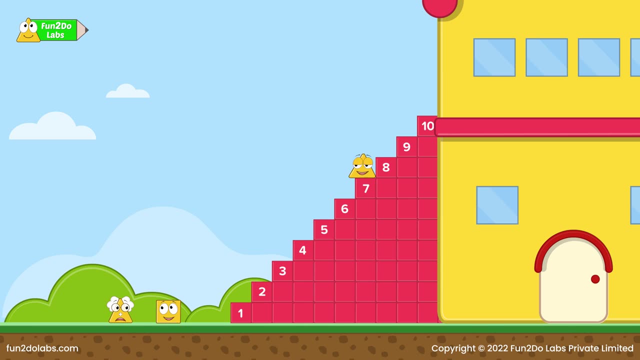 We count the steps as we come down. Together. they sing, dance and hop on the steps. Uncle Math, who was passing by, gets shocked to see the new steps. Oh no, what happened to the steps? Quickly, Trio and Squero narrate the entire story.